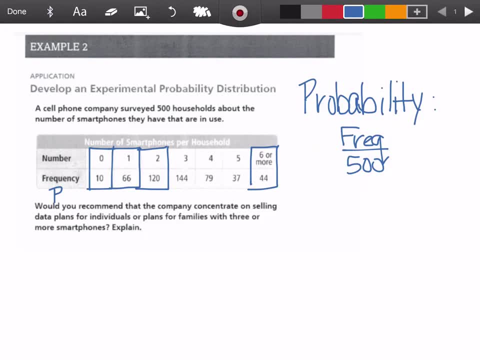 probability of each one of these numbers of cell phones being in use at one time of time. so to find the probability of zero smartphones being in use, we're gonna take the frequency divided by 500. so the probability of zero smartphones being in use is 10 over 500. so that's the probability of zero occurring, so 10. 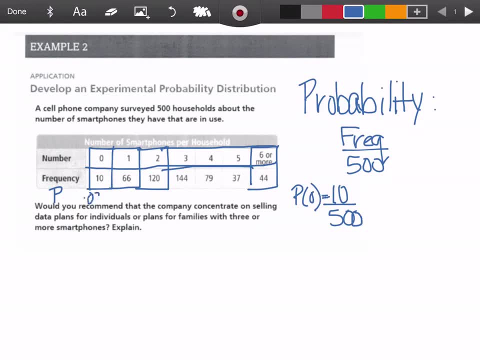 divided by 100 is 0.02. do the same thing with one. probability of one smartphone being in use is 66 over 500, and if we take 66 divided by 500, we're gonna have 0.132. so then we keep going and we keep doing this for the whole entire chart. so 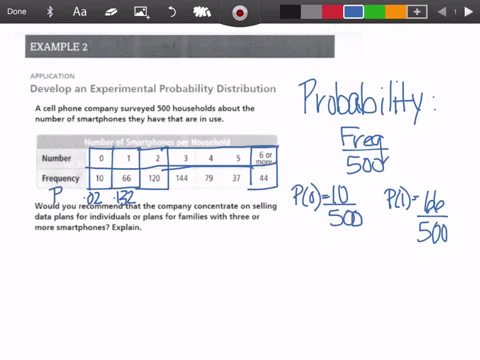 you can pause your video and those following probabilities and then check your answers with what we have. so now check your answers. you should have probability of 2 being 0.24. probability of 3 being 0.288. probability of 4 is 0.158. probability of 5. 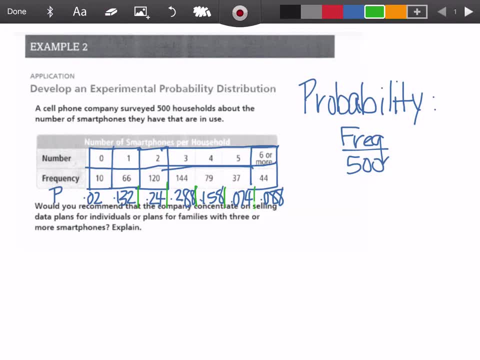 smartphones being in use is 0.074, and then the probability of 6 or more is 0.8 or 0.088. so would you recommend the company concentrate on selling data plans, plans for individuals or plans for families with three or more smartphones? 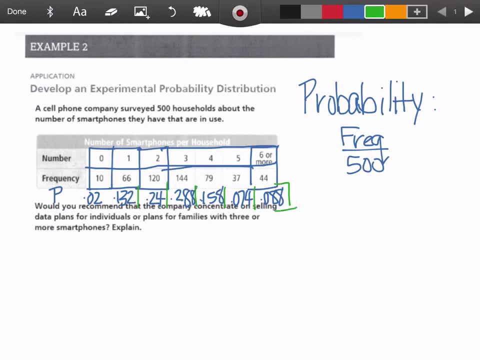 so to figure that out, we want to figure out which probability is more so, which probability occurs more often. is it going to be three or more people or less than three? So let's find the probability of three or more. So the probability that a family has three or more cell phones in use is the probability of three or four or five. 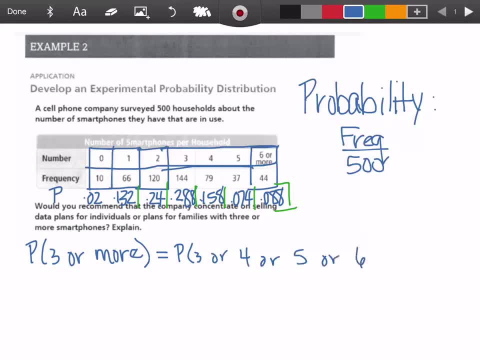 or six or more. Okay, notice how six or more that probability is going to be the same. That's going to be 0.088.. Remember that anytime you have probability with or we can add those probabilities. So we actually have probability of three plus probability of four, probability of. 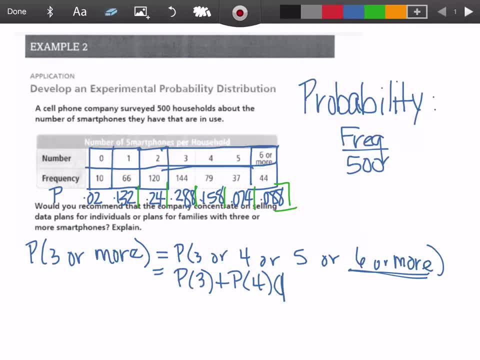 five. We're going to add that. So plus probability of five, plus probability of six or more, So I'm just going to say greater than six. So let's take all those probabilities and add them. We have 0.288 plus 0.158.. 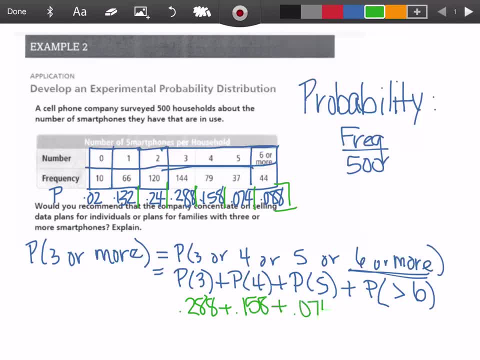 Plus 0.074, plus 0.088.. And adding all of those up, we get 0.608.. So that means that 60% of its consumers, which is more than half the consumers, are in the category that they have three or more. 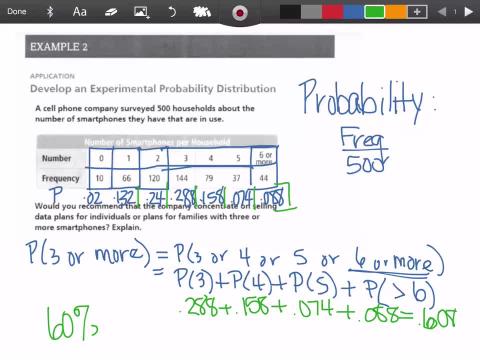 cell phones being in use At one time. So we want the data plans, or at least the cell phone company should have the data plans focused on families with three or more smartphones, Because that's more than half their company using that amount of smartphones. So now let's go over the next example. So we want to know: 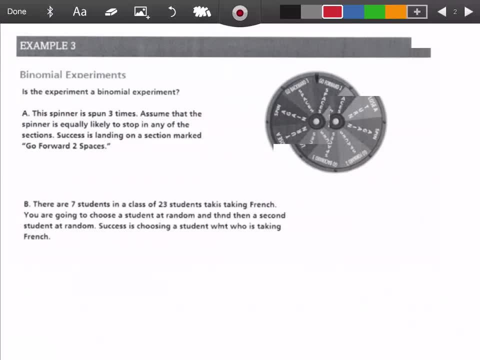 if this is a binomial experiment. There's two different examples here, Example 3A and Example 3B. Example 3A has this situation. This spinner is spun three times. Assume that the spinner is equally likely to stop in any of the sections. Success is landed on a section marked go forward two spaces. 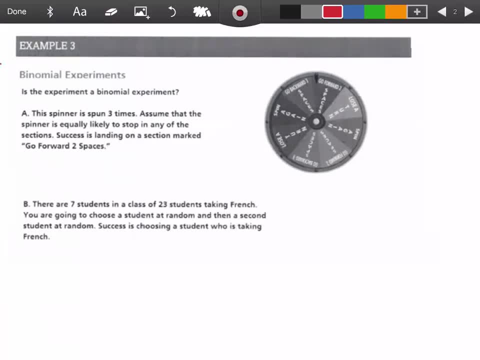 So, looking at this, our spinner has go forward two spaces at the top here and go forward two spaces here. It's very difficult to read, But some of the other sections have lose a turn spin again, go forward three spaces, So the only two that have go forward two spaces. 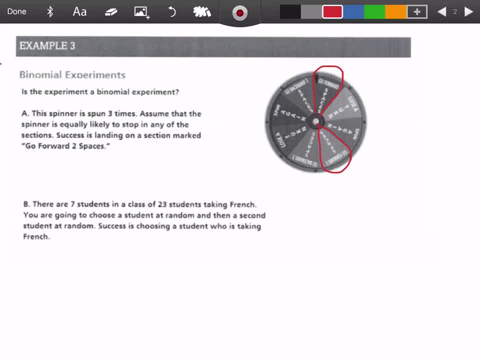 Are these? following that one circled and red. So is this a binomial experiment? That's what we're trying to figure out. So we have to remember what we know about binomial experiments. Binomial experiments have to have independent events. So if we think about this, Are these independent events? Do you spin once And then does it occur on your own? Look at this space travelled. it is going to do is be a independent feature. so that's the way to ask of temporal ASss, lobbying, assessment, maybe to blind or the date, Huh, but if they think about it. but they've got to use an optimistic way than the familiar. capabilities, then that's not the true pillar. So how will we know which is the closest value? Have these seconds in practice, theory, when you are Dáuné тоб la gηrna dùrılděούs, We will go the same question and everyytes. 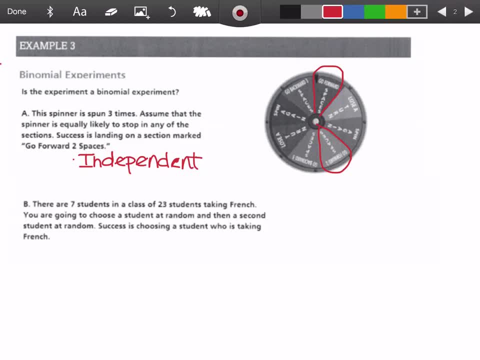 affect the second spin? And in this case no, because the spinner. we're not taking any portion of the spinner away. This is independent events. So you spin it once, it's equally likely to land on any section. You spin it again, it's still equally likely to land on any section. So we do. 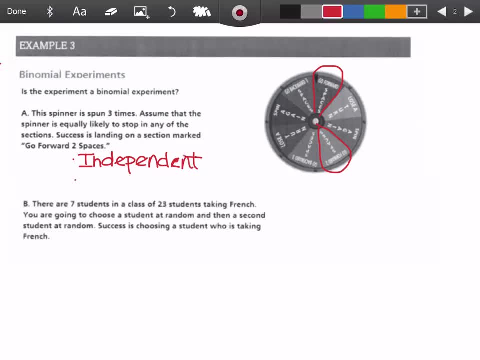 have independent events. I just said that it is equally likely to land on any of the spaces. And then another condition for binomial experiments is: are there only two outcomes? So we have to think about this one. Are there only two outcomes? 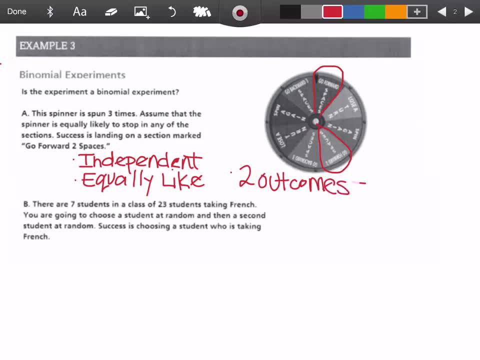 And it seems like there's multiple outcomes. because you could spin the spinner wrong. You could spin the spinner right. You could spin the spinner wrong. You could spin the spinner wrong And you could spin the spinner right. You could spin the spinner wrong And you could spin the spinner. 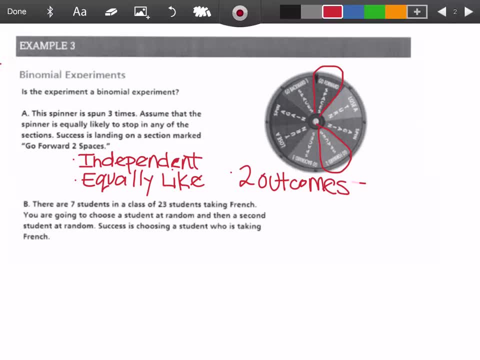 and land on, lose a turn, go forward two spaces, but two outcomes, meaning one is a success and one is not. so in this case, two outcomes. or this spinner does have two outcomes, the first outcome being: you land on it, so you land on what you want. the second, second outcome of a failure is: you don't land on it, you don't land on the. 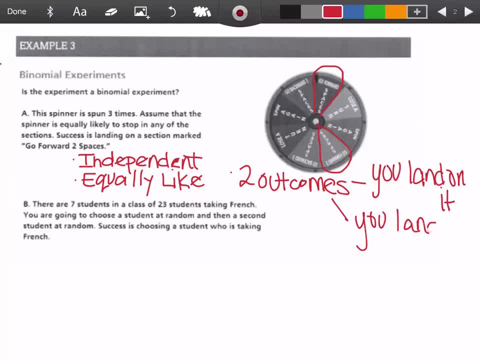 portion of the spinner that you wanted. so this is a binomial experiment. and just to talk about the binomial experiment, and just to talk about this one a little bit further, let's try and figure out what is the probability of success. so what's the probability that you do land on? go forward two. 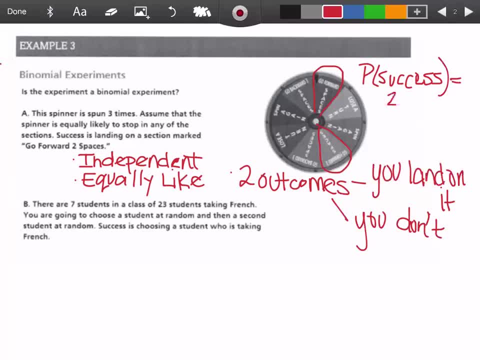 spaces. well, there's two sections that say: go forward, two spaces, spaces out of eight possible out of eight possible sections. so reducing that the probability of success is 1, 4th or a 25% chance that you're going to land on the section you want. so now let's start about example. 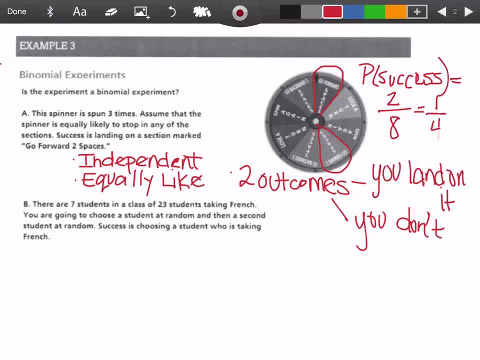 3b, there are seven students in a class of 23 students taking French. you are going to choose a student at random and then a second student at random. success is choosing a student who is taking French. so that's what our success is going to be called. but if we think about this one, 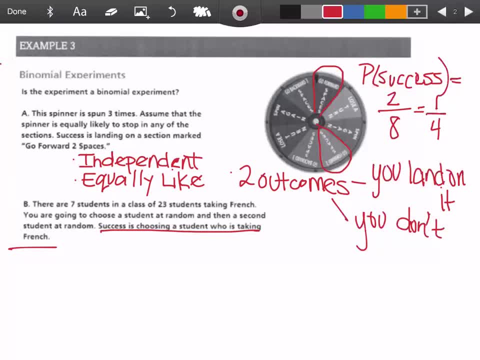 we need to know if we have independent events or not, and in this case we don't. we don't have independent events because the probability changes in the second pick- the first pick- affects your probability of picking a French student in the second pick. so probability changes on second pick.